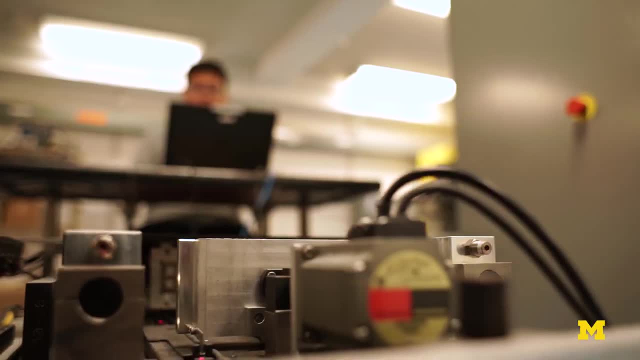 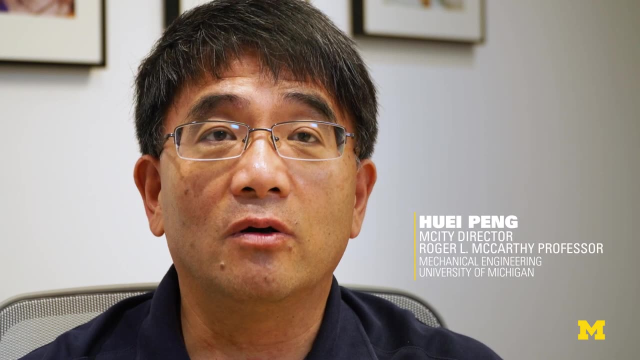 I want to see U-M play a central role in bringing people back, because we are providing technologies, providing know-how, and also our students. Mechanical engineering has played a very important role in maintaining our leadership in the field of automotive engineering for a century. 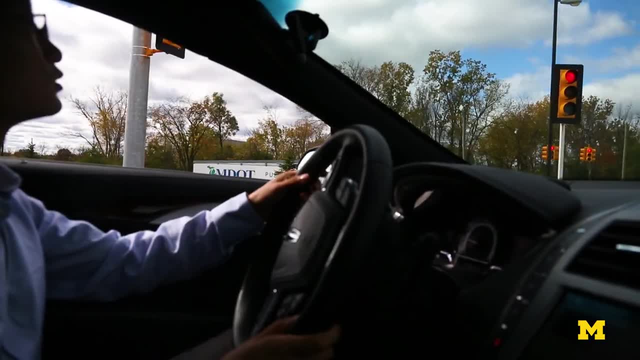 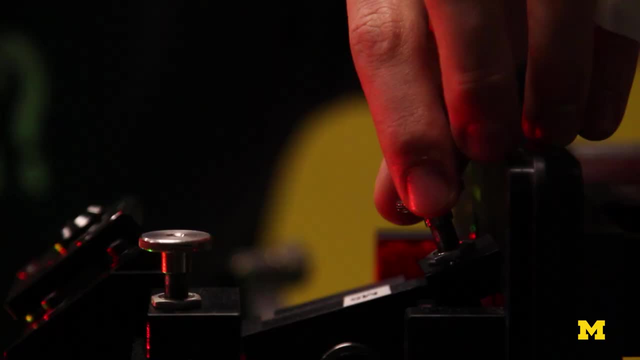 Still, they need to be safer, more efficient and less polluting. The fundamental principles that we teach in mechanical engineering are the following: The fundamental principles that we teach in mechanical engineering are the following: The fundamental principles that we teach in mechanical engineering were founded on energy transfer processes and we're trying to move those to. 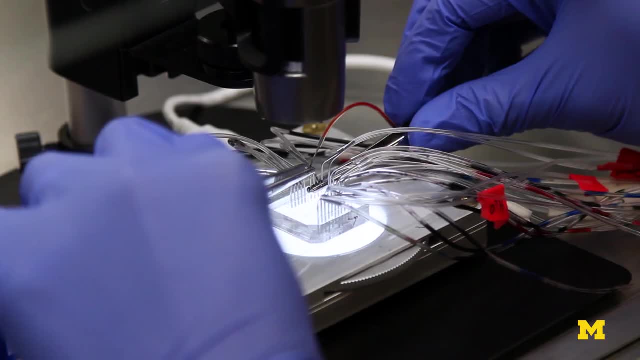 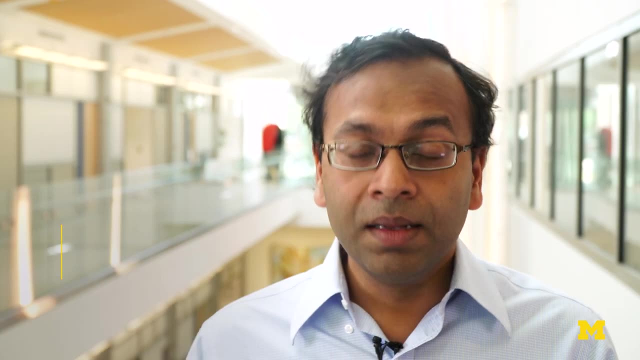 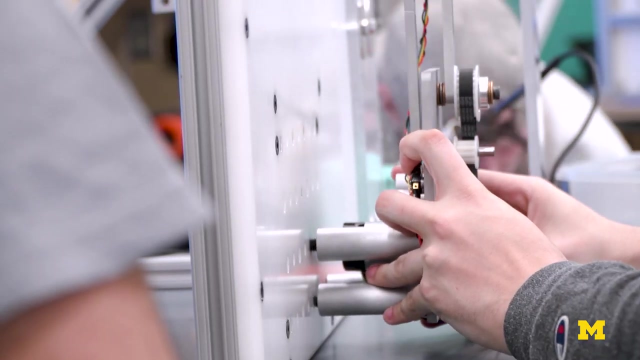 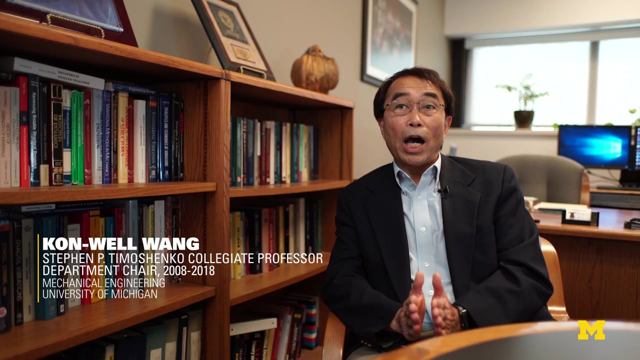 more sustainable and renewable energy carriers. We can apply principles of mechanics to address key questions and challenges in biology and medicine. Design and mechanical engineering at the University of Michigan has been an area of leadership for us. We've been pioneers in research and implementation of design. One main focus of our research is: we want to do high impact research. 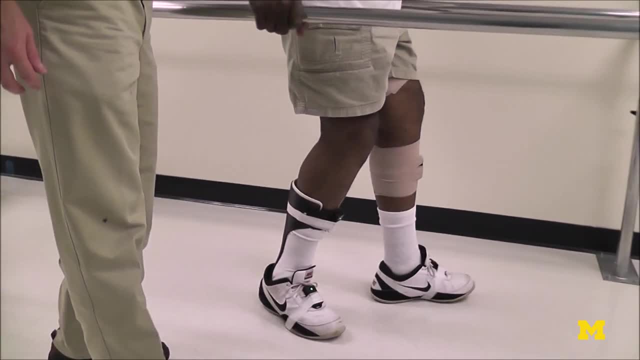 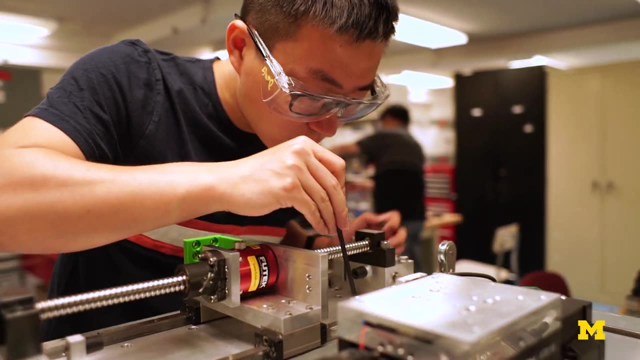 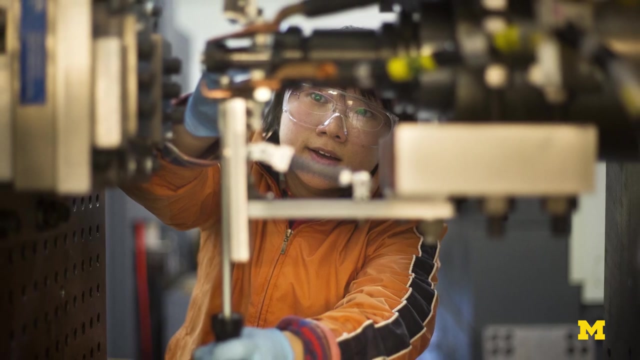 Now high impact to science as well as high impact to the society. We have faculty who work on the additive manufacturing processes, trying to improve them, trying to take them to the next level in terms of the quality and the types of materials that you could use for manufacturing. We have people working on smart manufacturing, really trying to leverage 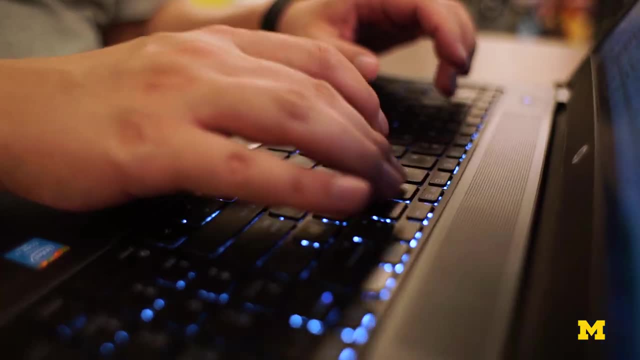 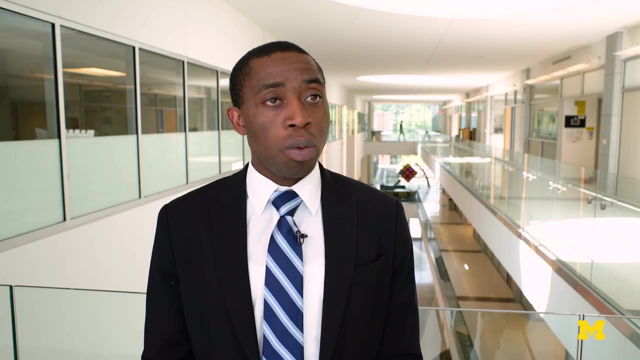 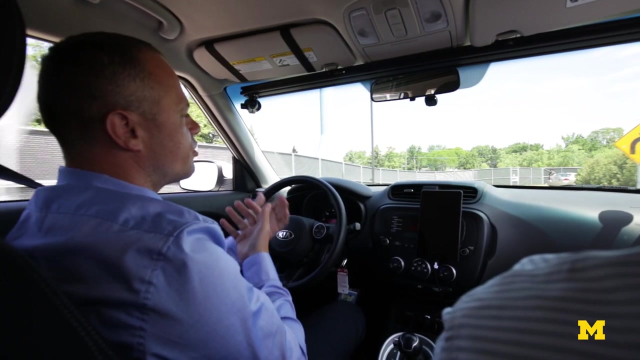 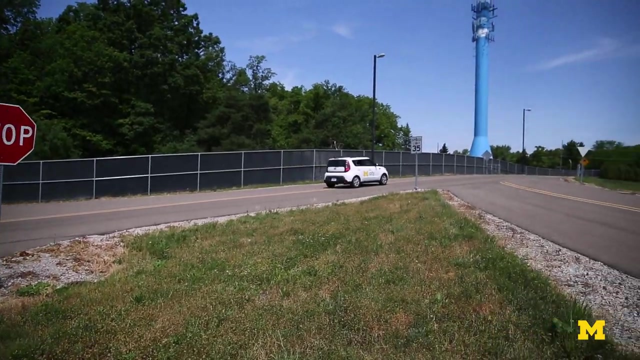 21st century technology, especially in the IT sector. Things like data science, artificial intelligence, bringing them to bear on manufacturing to improve profitability, improve throughput, Computation, communication, control- are at such a point that we can fundamentally change how cars are operated. With all these new technologies. they can be augmented by a robot driver, either working. 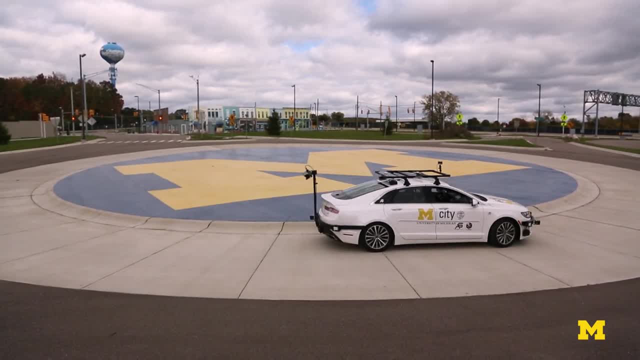 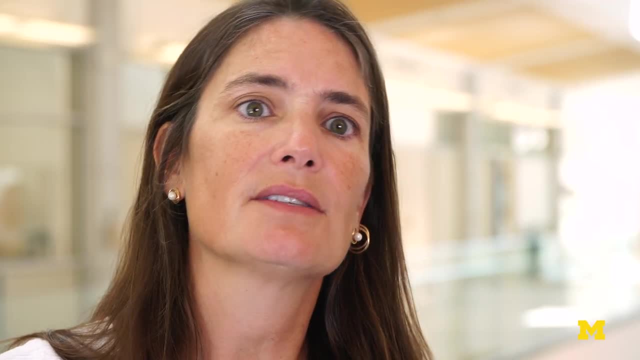 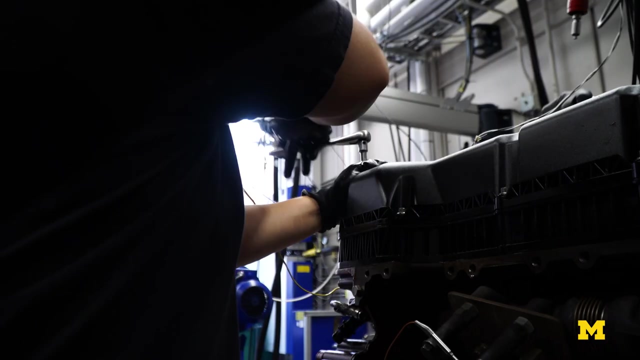 side by side with a human driver or completely taking over the control in certain cases. The energy sector is incredibly dynamic and changes from year to year, so we have to stay current. There's a clear demand from the students to be educated on this really critical issue. We've brought on new faculty that have research. 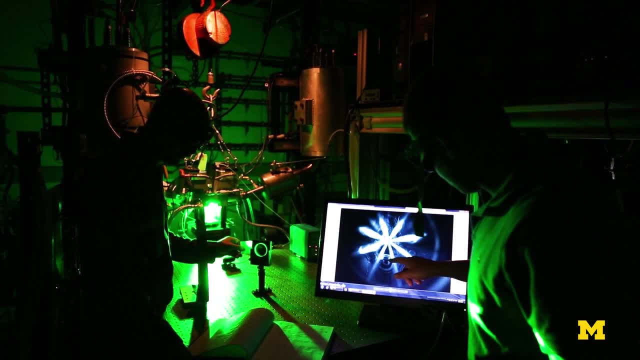 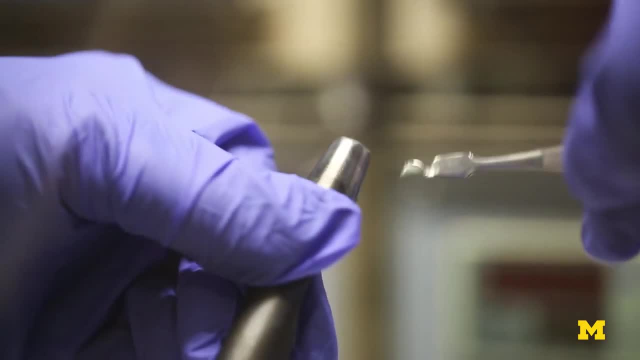 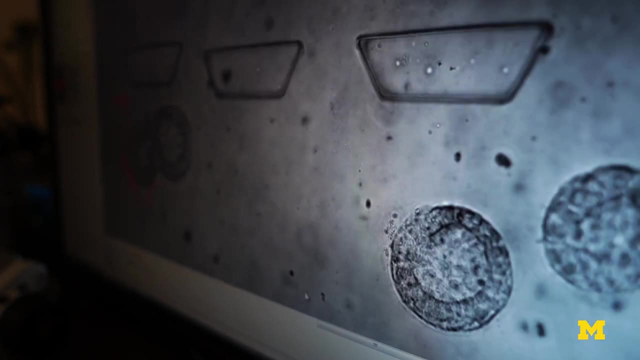 in other core areas of sustainable energy, which includes alternative fuels, sustainable fuels, but also, importantly, includes wind energy, solar energy and other renewables. We have been interested in mechanical biology. Basically, it's how cells interact with the surrounding environment. Then we also have 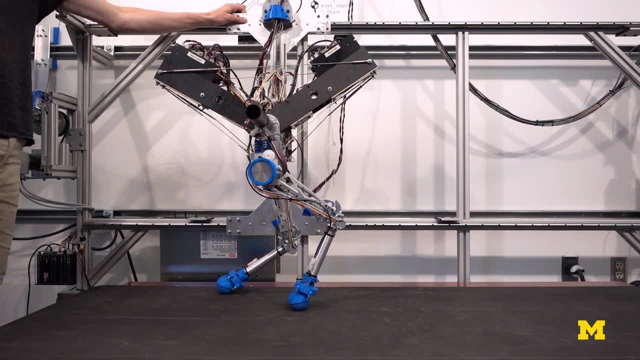 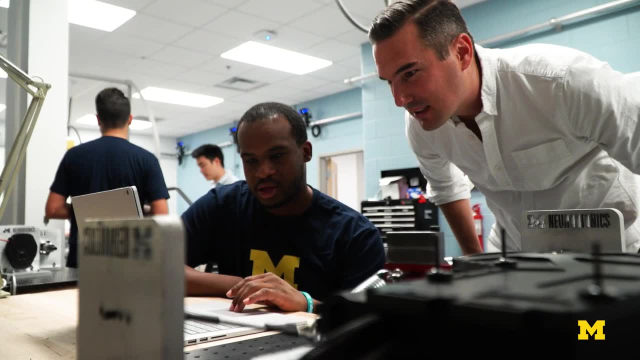 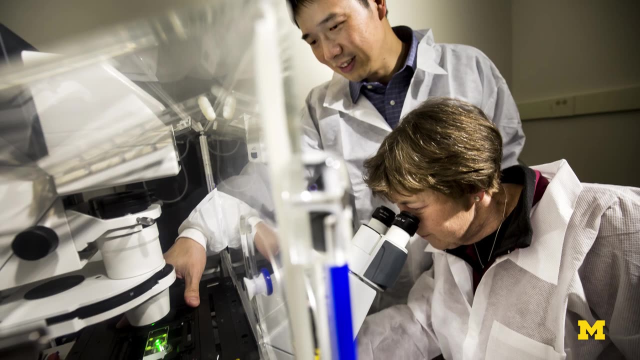 FACT members working on tandem mechanics, bone mechanics, rehabilitation robotics- So there are a lot of FACT members within this department. We're working very closely with people in medical school and biology departments and tackle some key questions. Going forward, mechanical engineering intends to remain the leaders in the field of design. 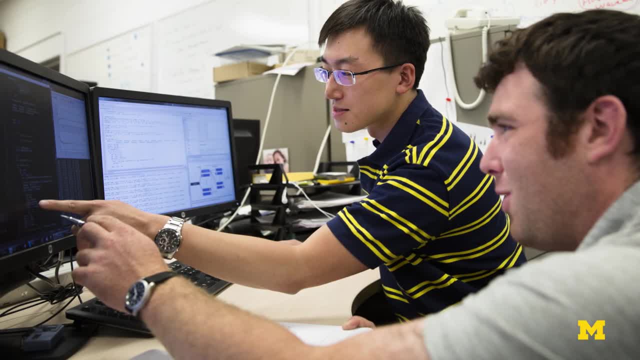 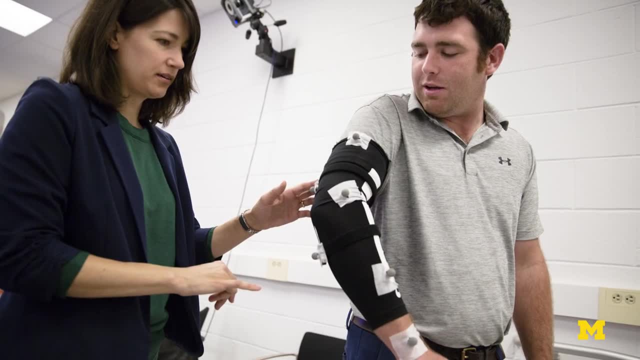 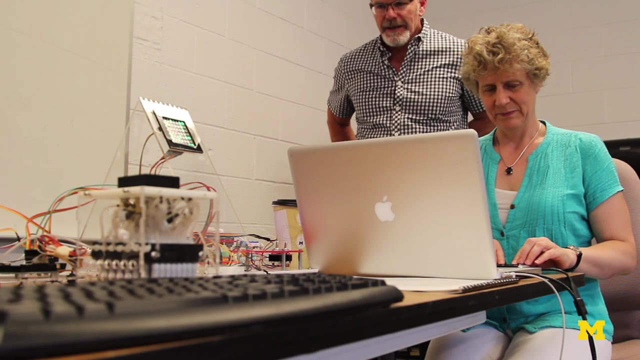 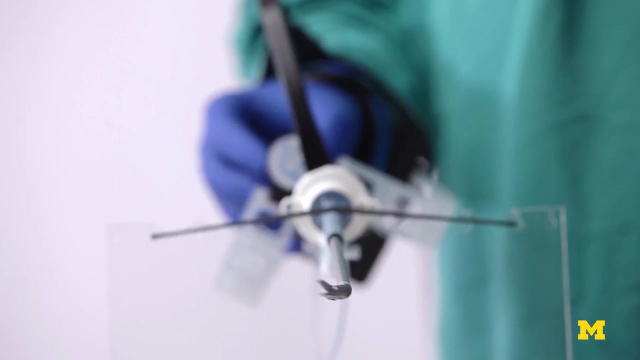 in particular, by conducting research and remaining at the forefront of identifying where the customer needs to be, what the customer's societal needs are, how to educate our students, giving them the tools to solve these needs and then, finally, developing an ecosystem that helps us translate our solutions to actual products that actually meet the needs of the society. 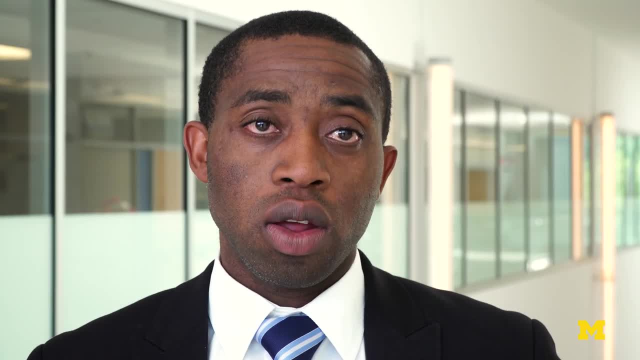 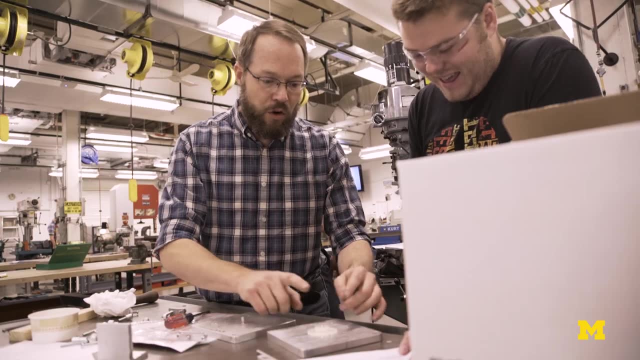 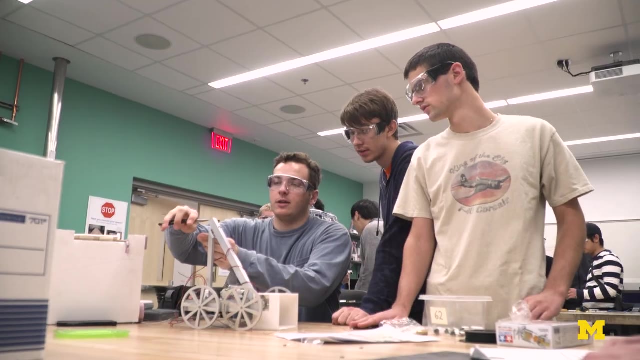 We have the benefit of our long-standing and excellent tradition and I think because of that we're drawing already the best students strong in teaching student fundamentals, that is, the mechanical science and mechanics. At the same time, we also have pioneered a curriculum that covers a series of team-based 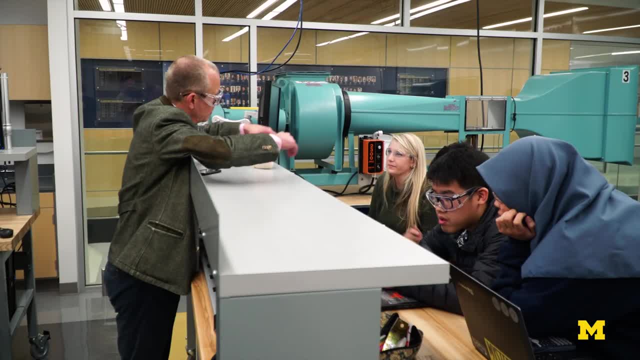 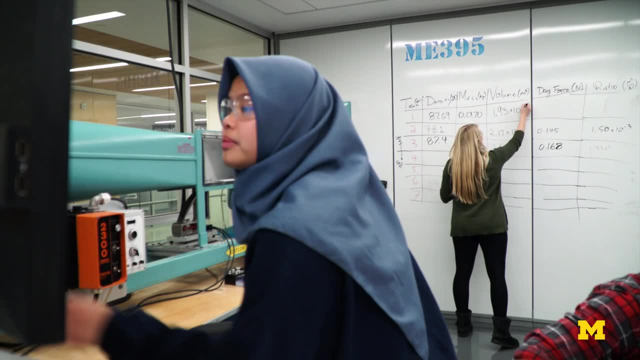 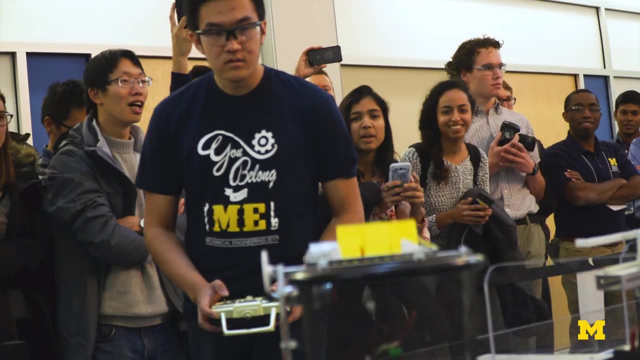 classes. The engineering education that we provide at Michigan and in the Department of Mechanical Engineering is meant to prepare students for a lifetime of contribution and service to the society after they graduate from here. At the same time, we want to make sure that we build diversity into our ecosystem here. 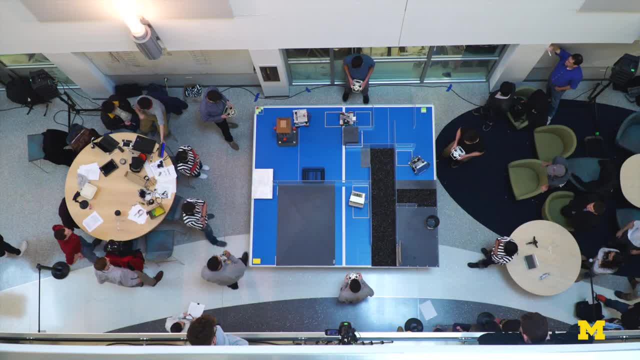 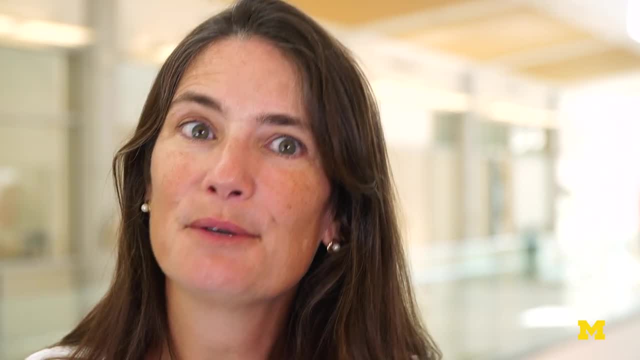 because intellectual diversity, diversity of perspectives, is essential as our students get trained to address these global challenges and global problems. We absolutely can't do it alone, and so mechanical engineers, as we train them, need to be able to interface with other disciplines. 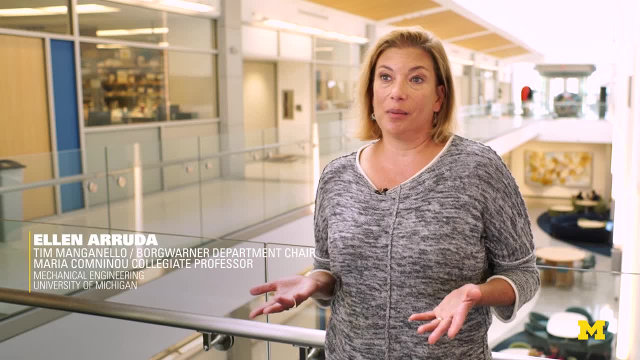 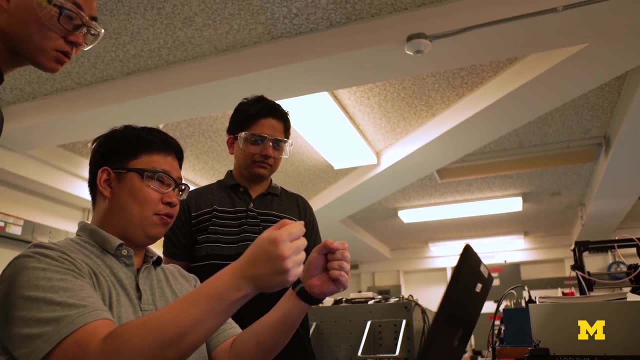 I love my job. I think a lot of my colleagues love their jobs. You know, I don't want a student to come here because somebody told them: you know you're good at math, be an engineer. I want students to come here because they're excited about engineering design helping. 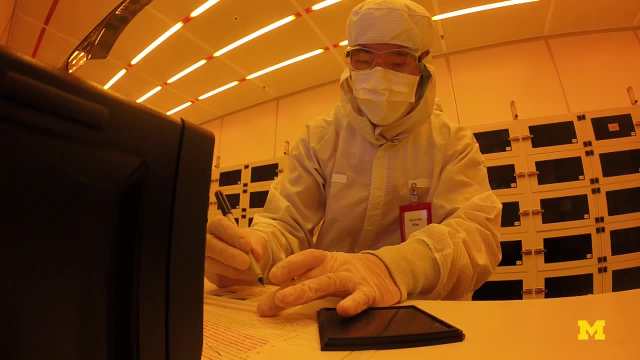 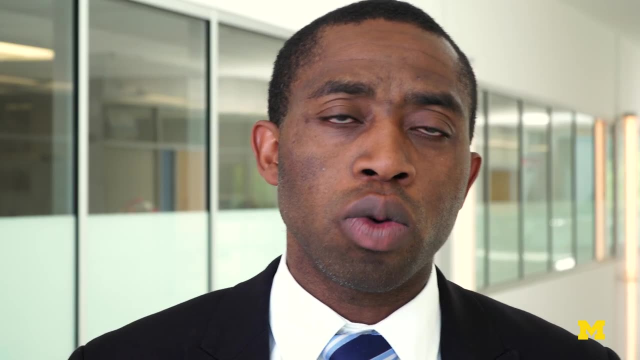 people. solving the world's problems, making society better. That's what engineers do. We are not afraid to push our students to the limits, because we believe that they've come here, because this is an excellent place, and so we want to make sure that we make them. 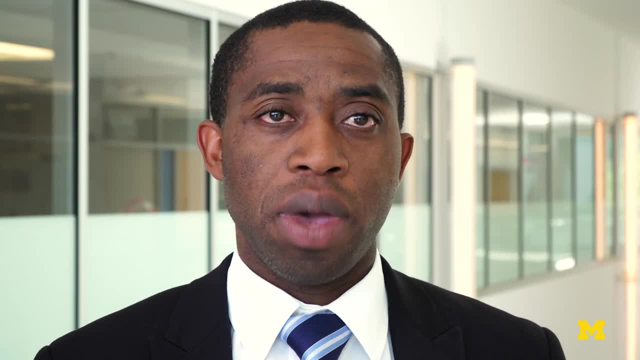 live here believing and knowing that they are the best of the best. Thank you, Thank you, Thank you.